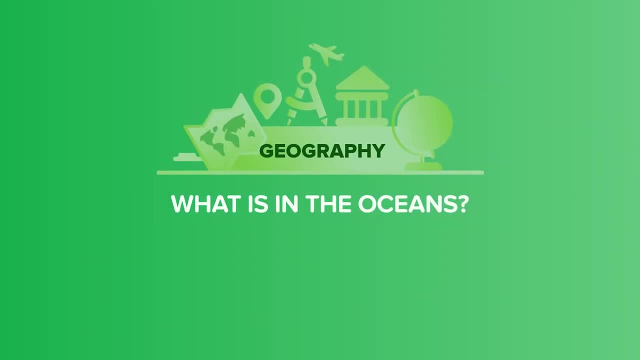 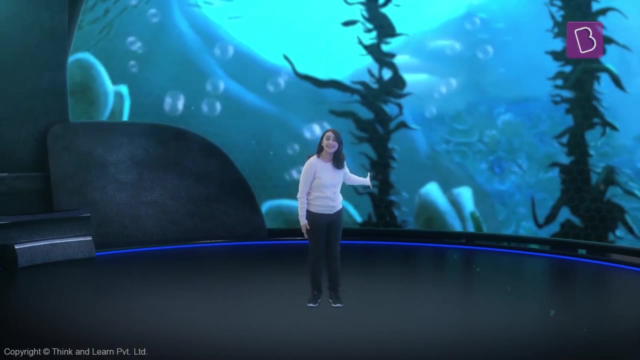 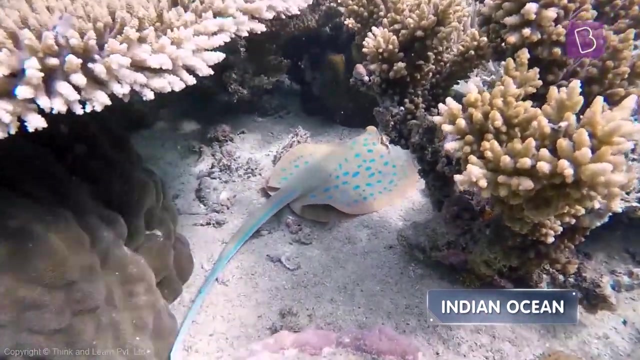 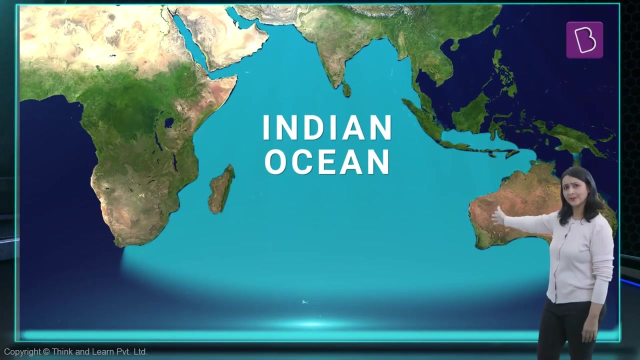 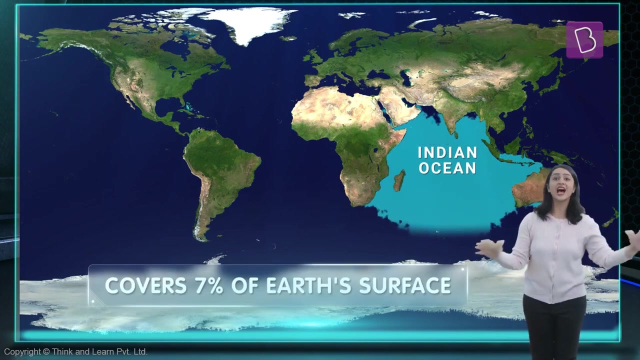 Welcome to the Indian Ocean. Isn't this amazing? Look at all these corals and sponges. Wow, Right now we're at the Indian Ocean Over here. This ocean is pretty large. It covers around 7% of the entire surface of the earth. 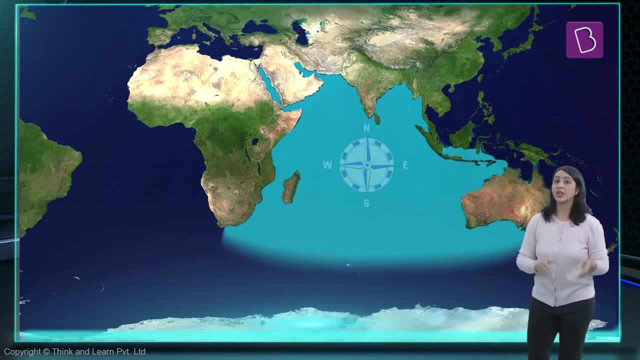 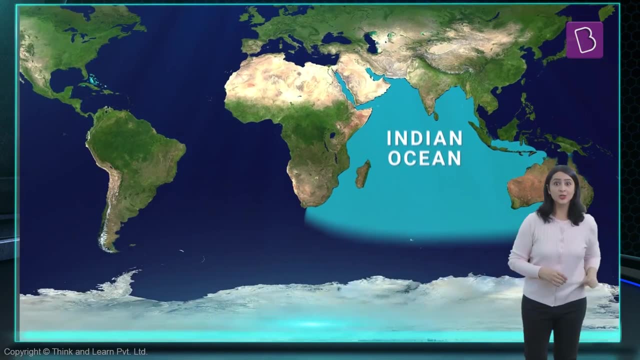 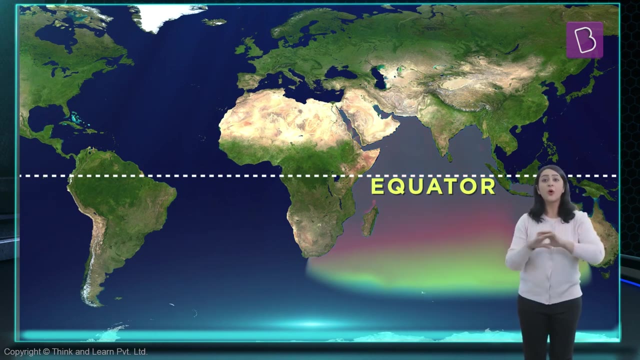 It's almost triangular in shape and it's got Asia on the north, Africa on the west and Australia on the east. Also, the equator passes right through the Indian Ocean, making it the warmest of all the other oceans. Now see this. 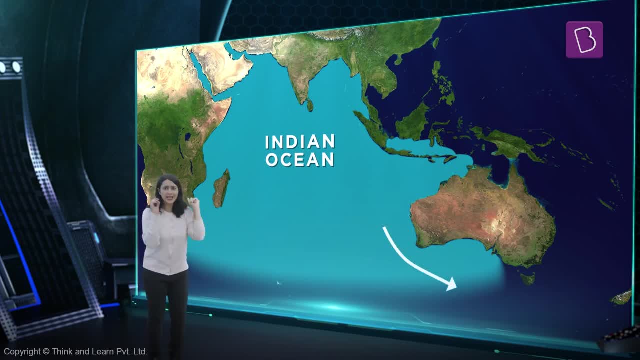 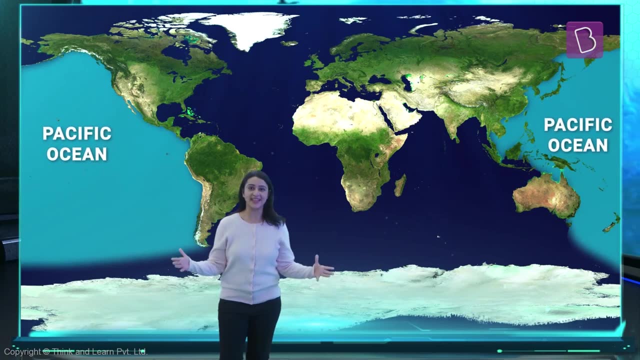 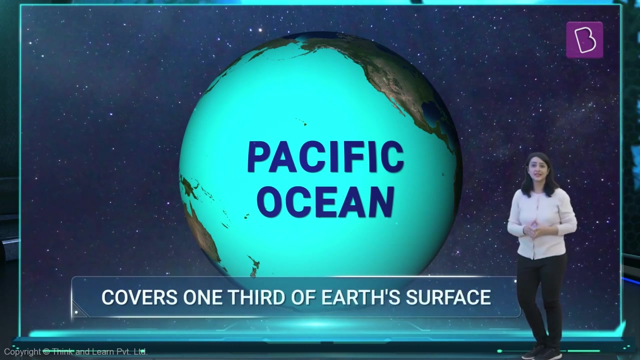 There's a moving channel of water around here. If I catch it, I could just ride it all the way to the Pacific Ocean. The Pacific Ocean, the largest ocean on earth. It covers more than one-third of the earth's surface and nearly half of earth's water surface. Can you believe that? 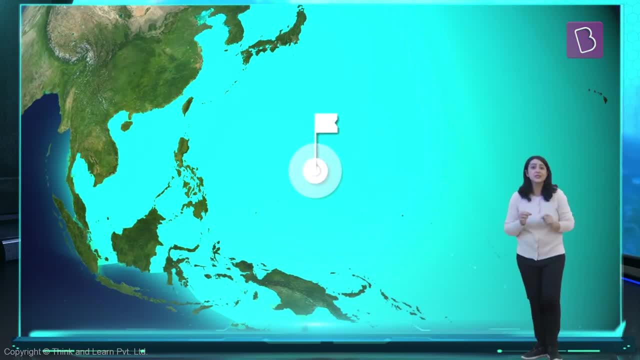 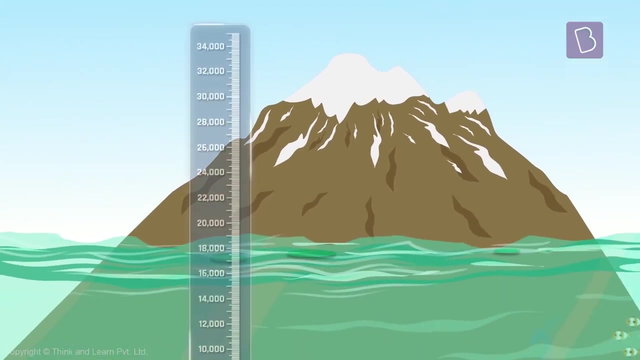 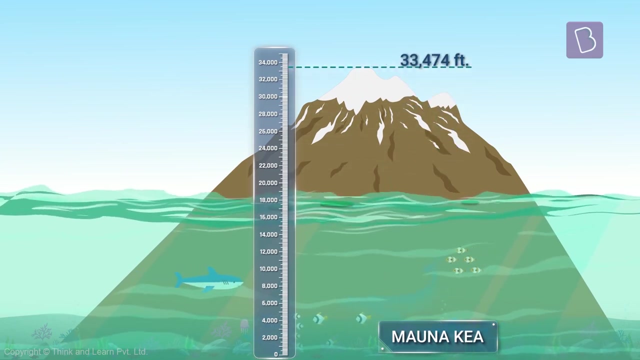 It's pretty deep too. It's got the deepest point on earth, which is called the Indiana Trench. The Pacific also has an underwater mountain near Hawaii called Mauna Kea. Did you know that it's actually bigger than Mount Everest, clocking in at 33,474 feet? Everest is 29,030 feet. As you can probably guess, this ocean has a lot of living things in it, So many that most of all our seafood comes from this ocean. I'm going to go through here, right between North and South America. 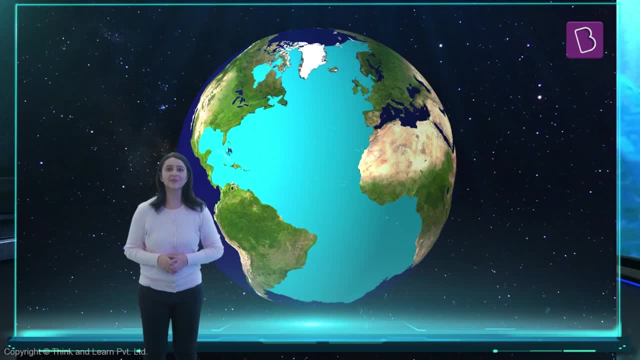 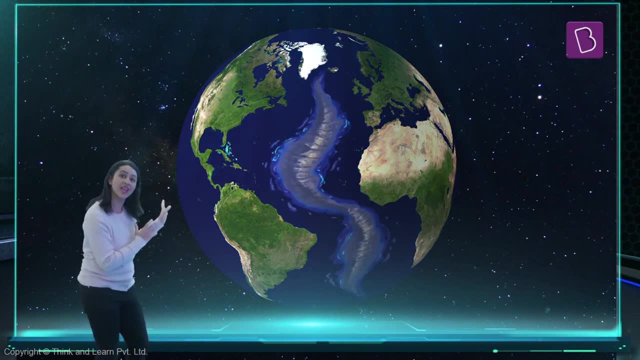 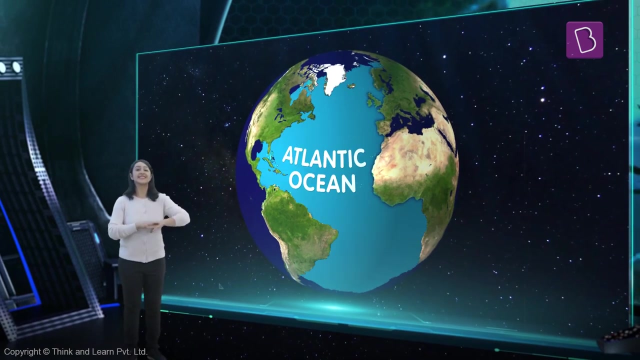 through a place called the Panama Canal. Welcome to the Northern Atlantic Ocean. Now, this is interesting. Look, there's a mountain range underwater here. The ocean is about an inch long, which is even longer than anything that you find on land. It's called the Mid-Atlantic Ridge. Now this ocean is the second largest in the world. 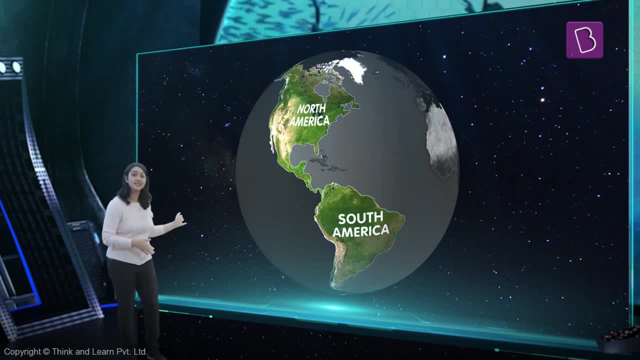 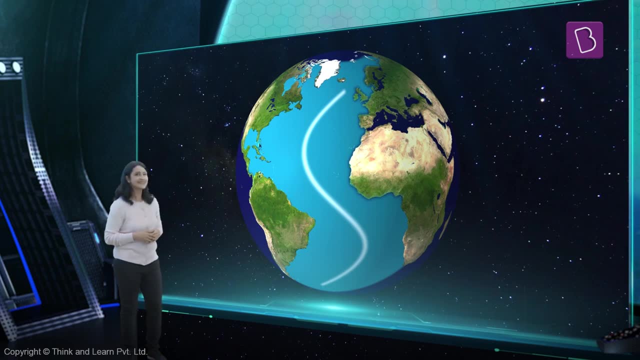 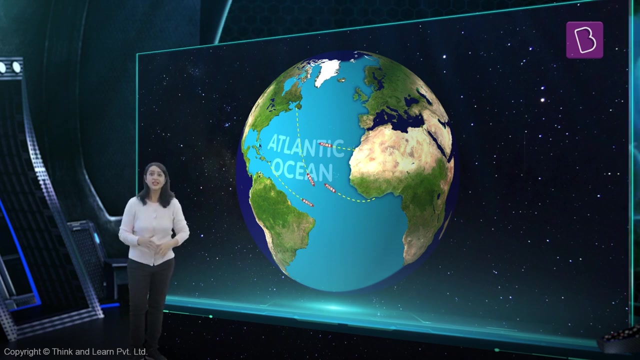 It stretches all the way from the Americas on the West to Europe and Africa in the East, almost forming an S shape. Now there's a lot of business activities happening on the port, So let's take a look at the ports of this ocean, because there are so many ports along the coastlines.